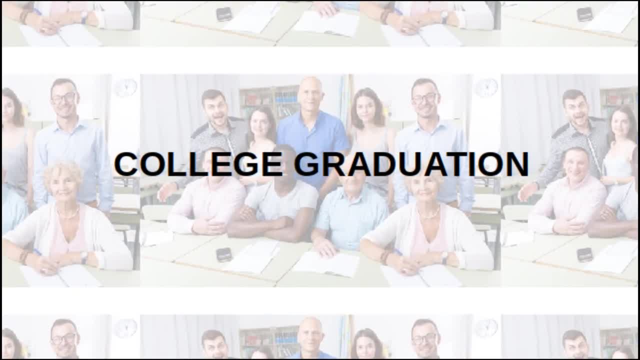 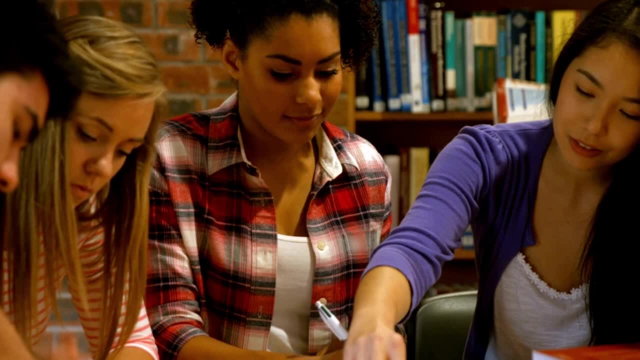 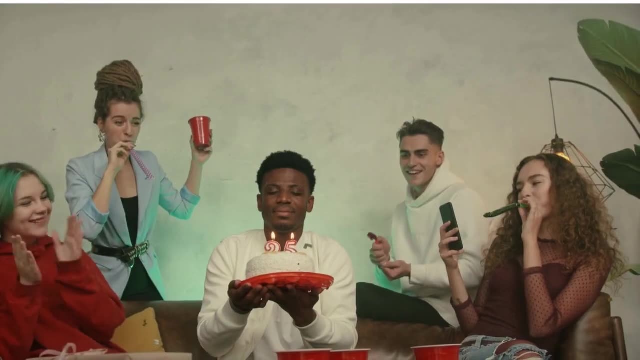 advantages to being an older college student, College graduation. Since there is a 30 to 50 percent of student population at most colleges who are over 24 years of age, almost everyone is likely to find at least a few college classmates. 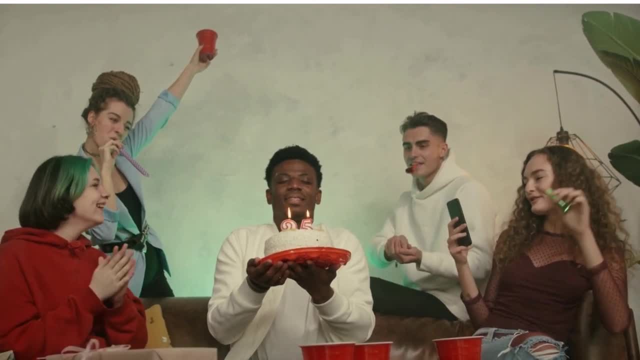 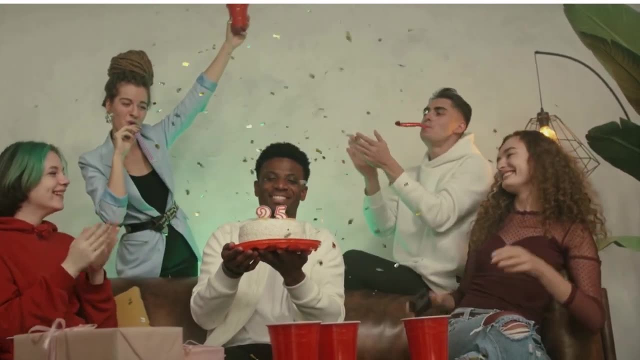 who are more likely to graduate college within four to six years of enrollment. The highest number of college graduates in a given year in the US are students between the age of 25 to 29.. This is likely because of a higher increase in enrollment of college. 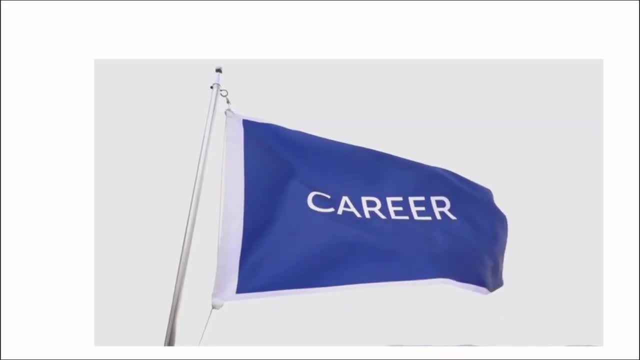 students age 20 to 24 years. Over a third of full-time traditional college students drop out in a few years and some others enter the workforce after high school graduation, only to restart college several times Several years later as independent students, Some older independent students of 22 to 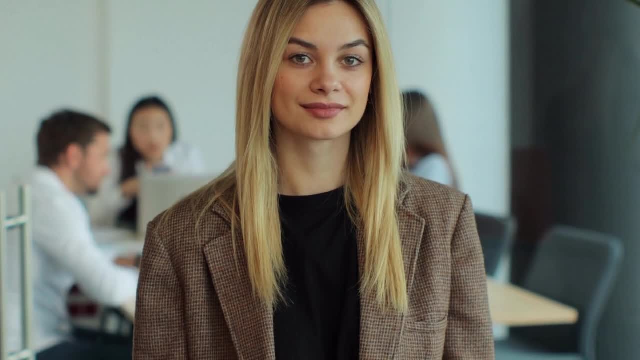 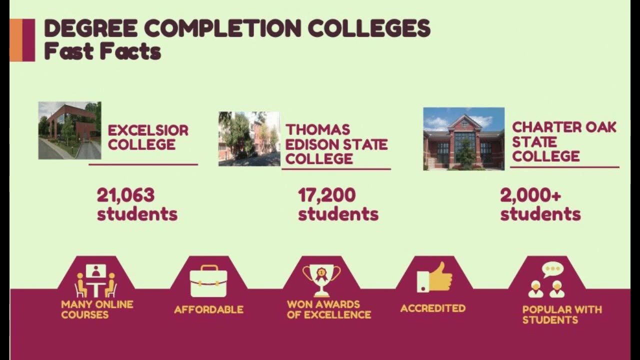 30 years indicate they have better career success and choice of college major upon delaying college by a few years. With the college graduation rate of 46.2 percent and many Americans 24 plus years with college credits but no college degree, there is a strong need for degree completion programs. 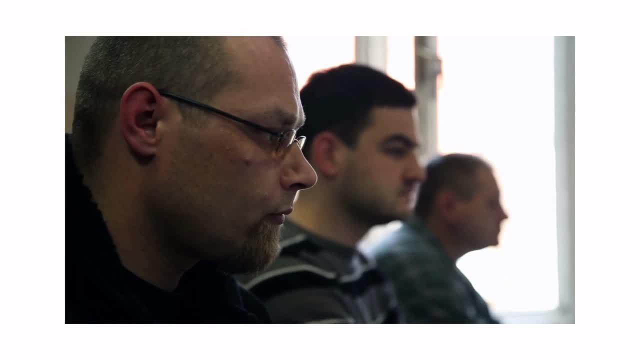 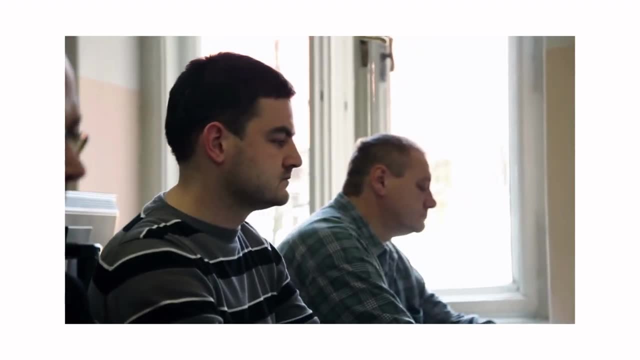 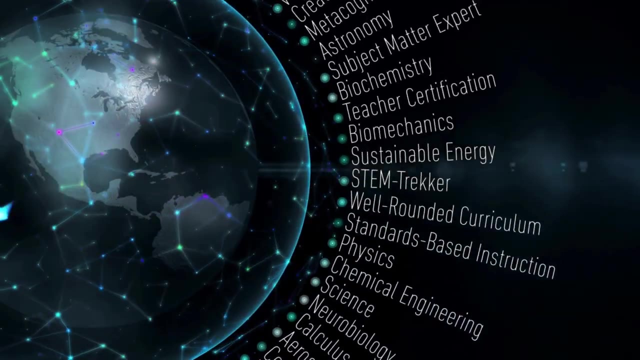 to quickly fill the gap toward graduation. A majority of students at the degree completion colleges, such as SUNY, Empire State, Excelsior or Granite State College, are over the age of 25.. Students enrolled for a bachelor's degree are more likely to complete college than 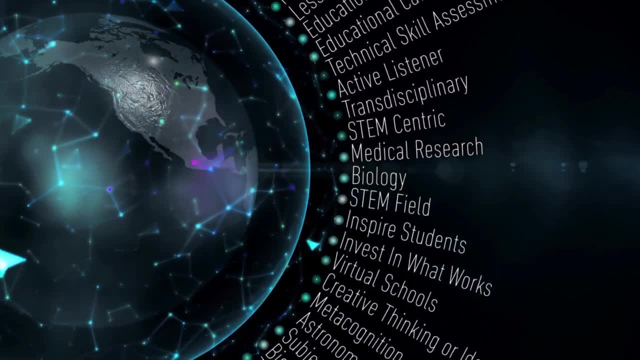 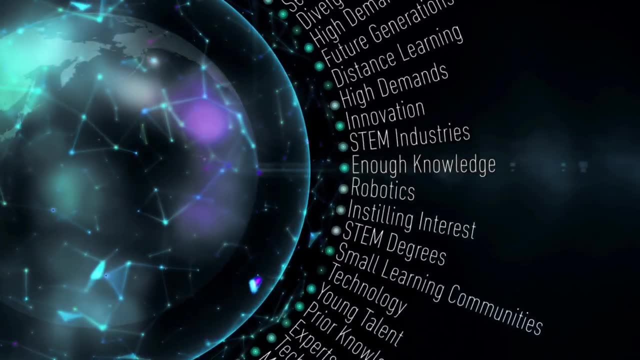 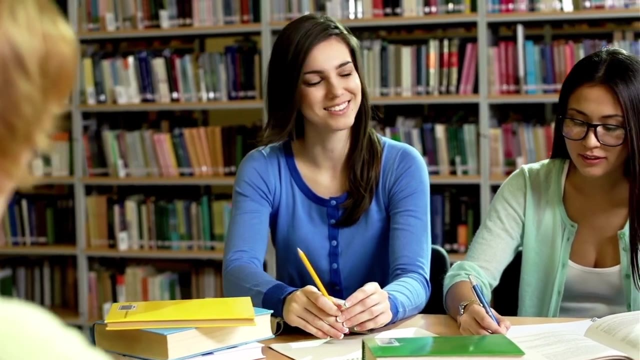 those who are enrolled for an associate degree. STEM fields- business and health care- make up a bulk of all majors for college students who graduate with a bachelor's or associate degree. The number of women enrolling and graduating college each year slightly outnumber the 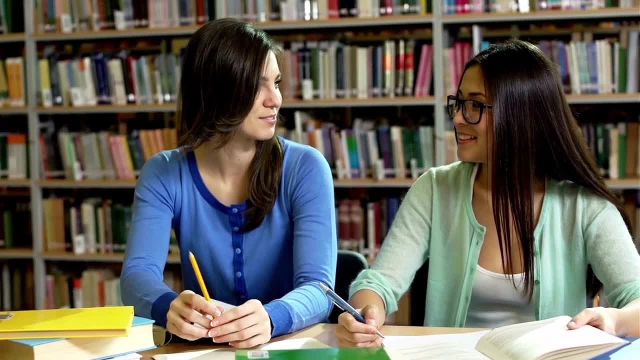 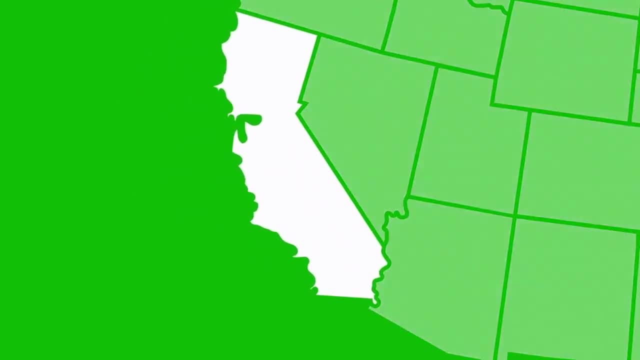 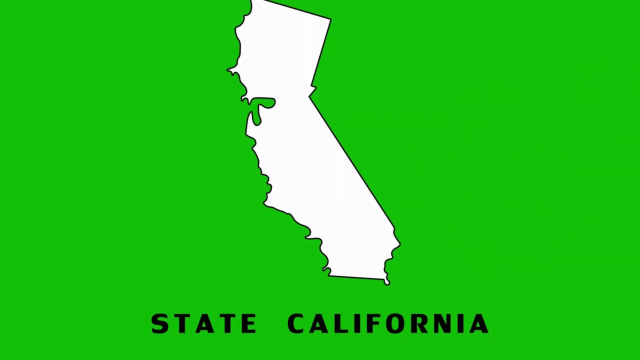 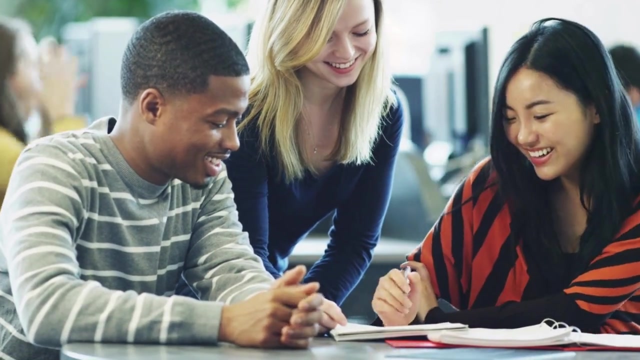 number of men enrolling and graduating college. Men make up the majority of engineering and computer technology related bachelor's degrees. In the US, California has the highest number of all college graduates, followed by Texas, New York, Florida and Illinois. Finding a college for your age preference: Having classmates in college whom you can. 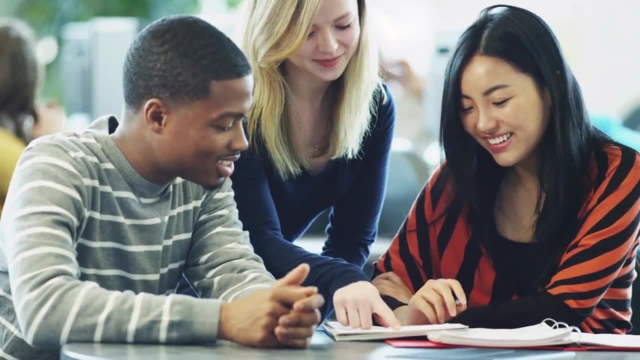 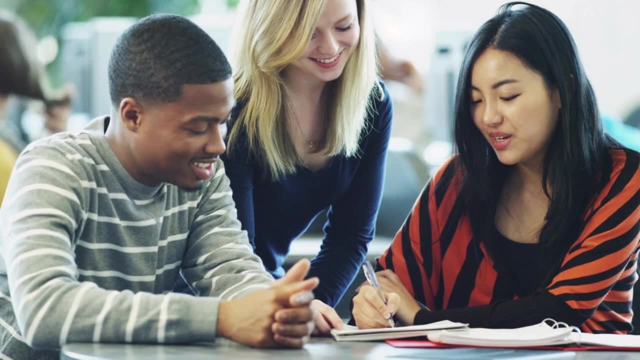 easily relate to and make friends with can be very helpful for a good college experience and for completing your college degree quickly and easily. So it is generally a great idea to find a college that fits your exact age specific needs. You might also have individual 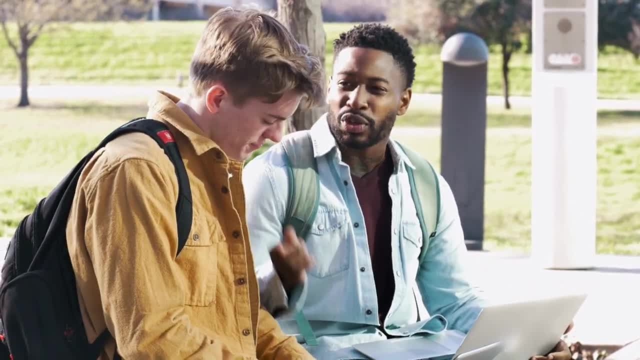 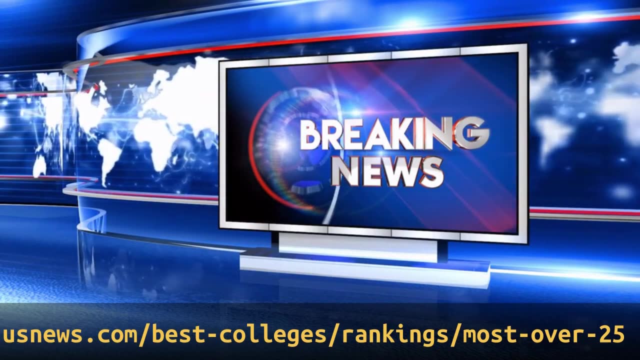 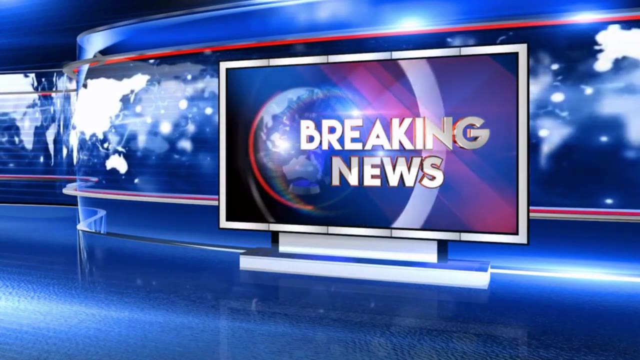 age preferences, which will help you get more comfortable with the college you enroll in. There is an excellent article from US News which lists colleges that have students over the age of 25.. The top colleges in the list have many older students and the bottom colleges in the list have more of the traditional 18 to 23 years of age students. So simply go through this list and find colleges for your age, plus and minus a few years. You can also contact the colleges directly and find out more from their alumni students for your preferred. 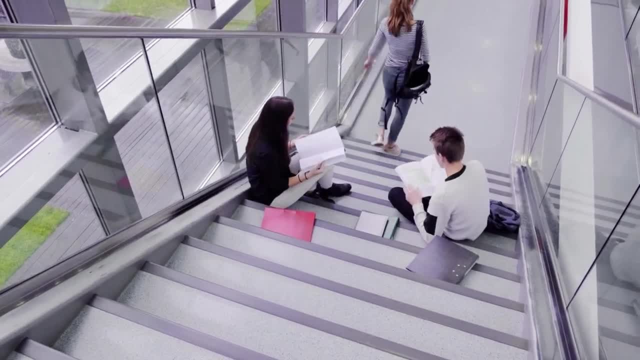 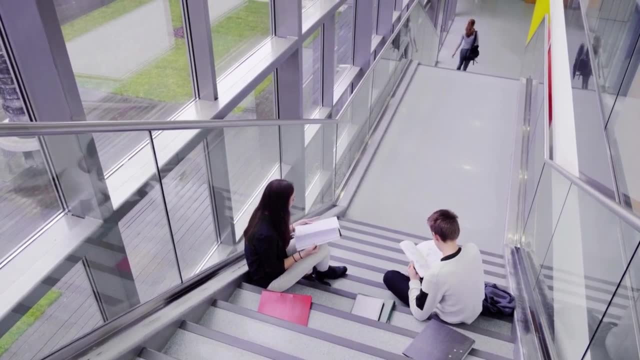 age group. If there are colleges near where you live, just visit the campus and talk to some of their students and they will help you find the right college for you, your students and ask them about the average age of their students. 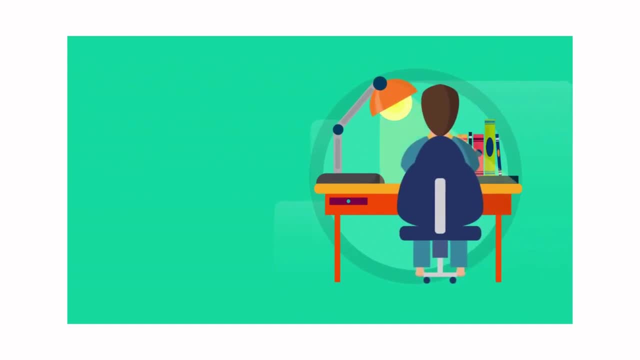 Faster College Graduation. Many college students assume there is not much they can do other than studying hard and scheduling more classes for faster graduation. But there are many other ways to quickly earn college credits, and such credits can easily transfer to most accredited US colleges. Here is a step wise Strategy for Quicker College Graduation ends and gives you an upfront understanding of how to quickly earned college credits, and such credits can easily, Very safely, transfer to most accredited US colleges. Here is a step wise strategy for quicker college graduation. 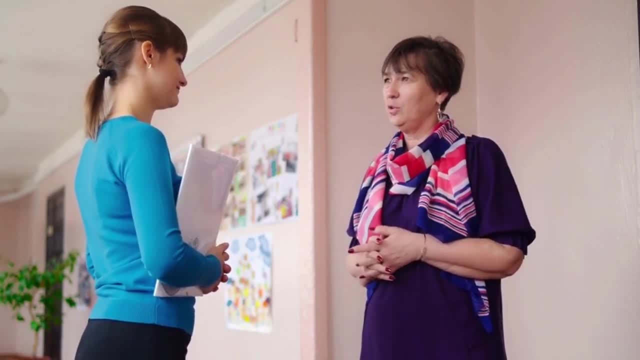 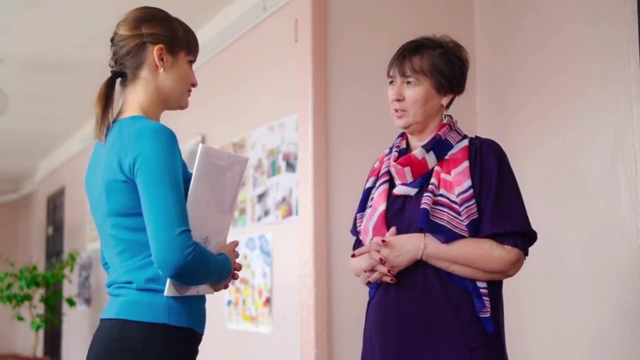 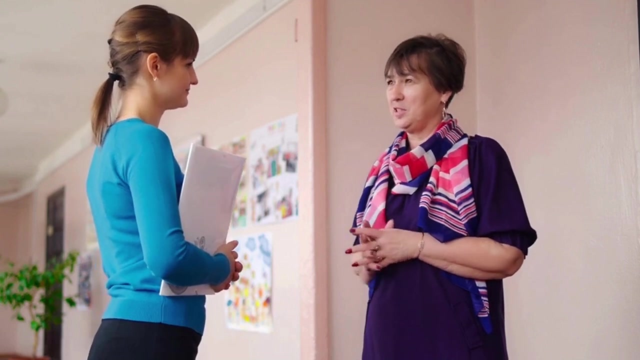 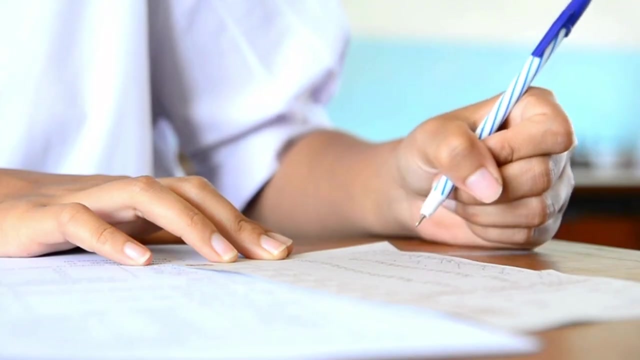 graduation. find out from your college student office about their credit transfer policies. also, ask senior students and anyone else in the know at your college about how to transfer in credits to your college. in case you find out your college does not accept much credits by transfer, consider transferring out to a degree completion college for your degree. most degree completion. 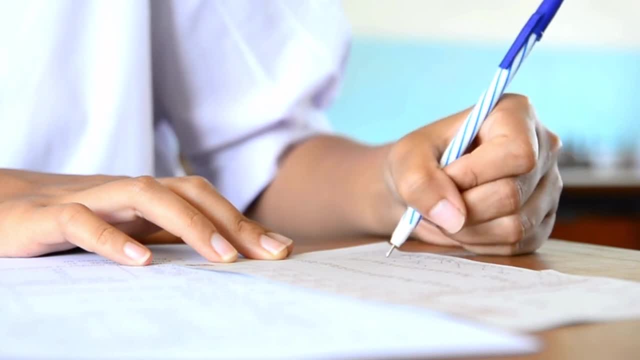 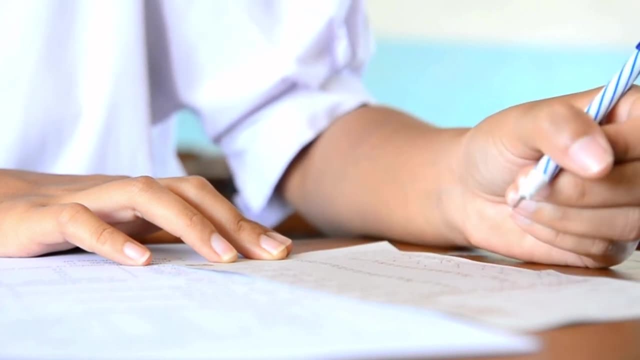 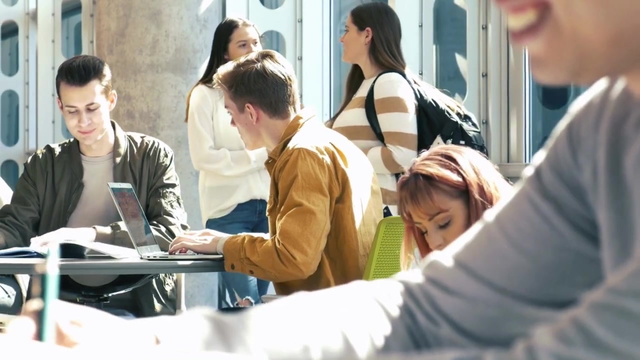 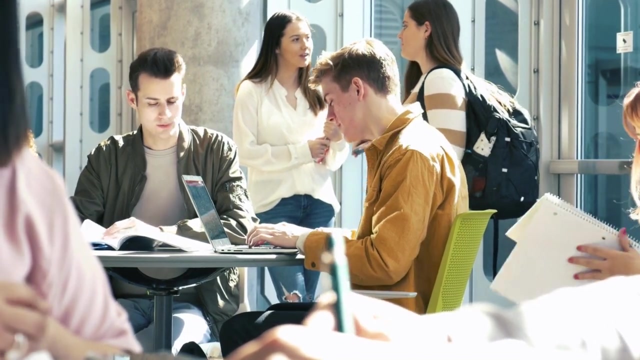 colleges are extremely transfer friendly and can easily transfer in all your previous college credits from other colleges, courses and standardized tests. write clip or dsst exams for some subjects that are part of your current degree curriculum. also sign up to instant cert for practice tests and flash cards for the test preparation. take any sailor or other ace or